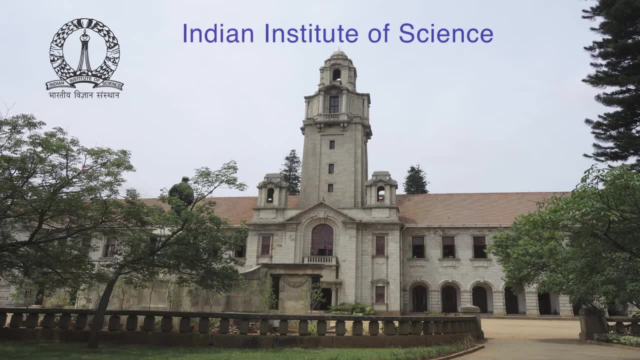 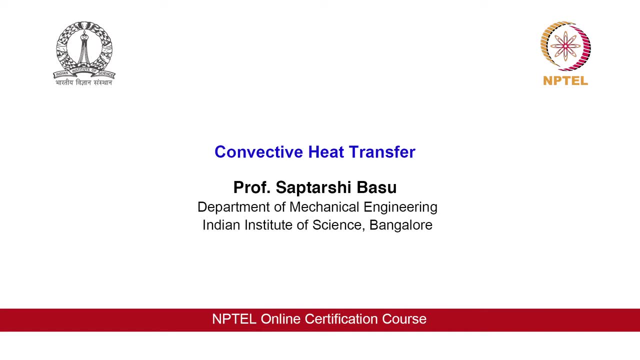 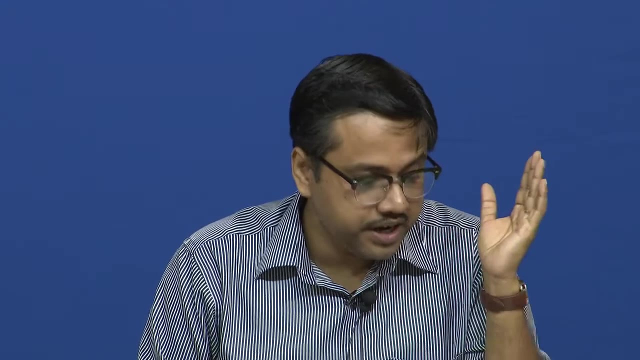 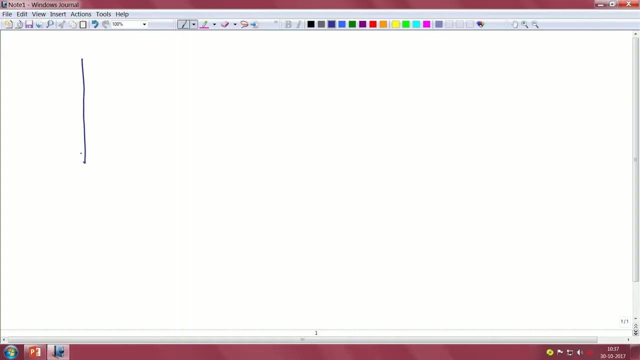 So in the last class, what we did was that we for understanding this thermal stratification- okay, if you recall the problem that it was still that vertical plate, okay, and one thing that happened was that the temperature of the ambient actually increased from T infinity 0 to some T infinity H, if you recall, okay, which decreases basically the heat transfer. 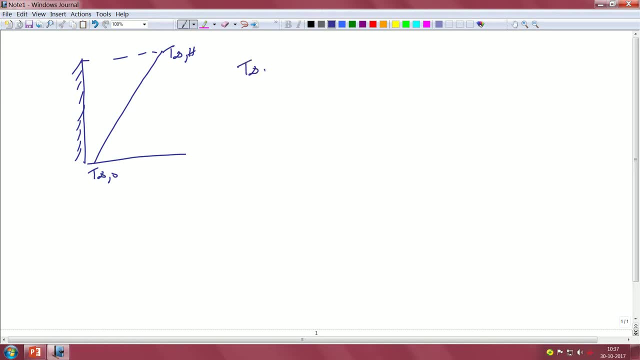 potential. okay, So this is obviously we said is going to be greater than this, right, and we defined parameters which basically convey the meaning of this. okay, So our definition, by our definition, Y was equal to Y by H. if you recall- just consult your notes- delta was normalized by H, R a H to the power of minus one-fourth, okay, V bar. 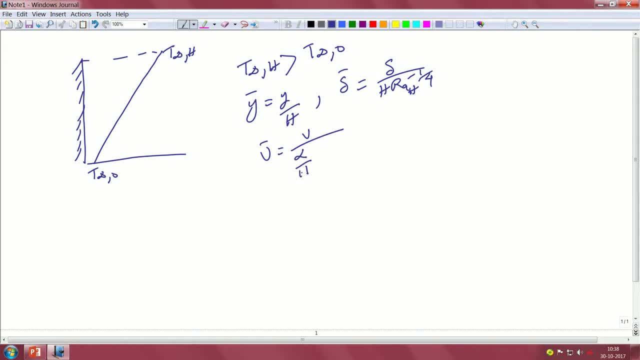 is given as V divided by alpha, by H, or is the number H to the power of half, okay, and B, which is basically signifies the what is the what is the increase in? basically the room temperature, okay, or the ambient, okay. So this is given by a non-dimensional parameter, B, where we said that as B goes up, the heat. 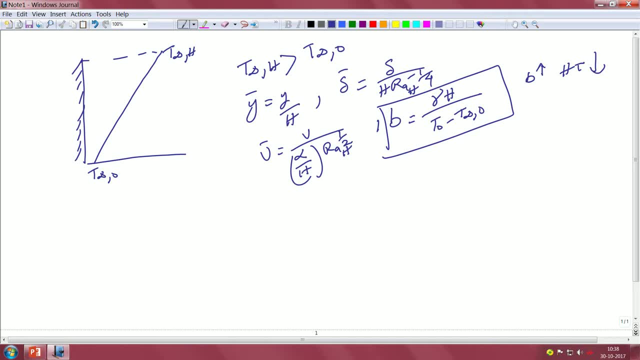 transfer actually decreases, right. So up to this point we did okay. Now we also cast the integral equations. okay, if you recall from last class that we ahh, cast both the energy as well as the momentum equation in integral forms. Now we substitute. substitute in momentum. 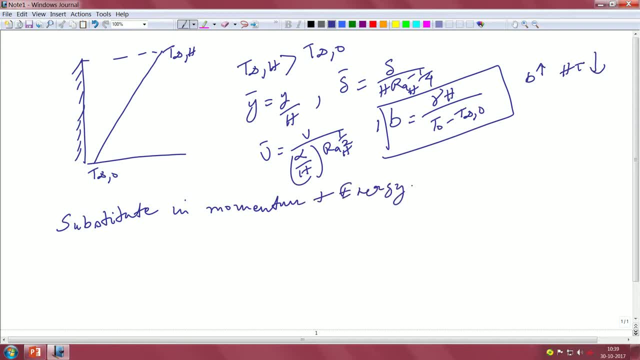 plus energy equations, okay. So, in a nutshell, what we get is: okay, Okay, Okay. So these are the expression. this is the first expression, is the momentum, obviously. then comes the energy equation, Okay. So these are the two expressions that we get, okay, and of course, your wall heat flux. 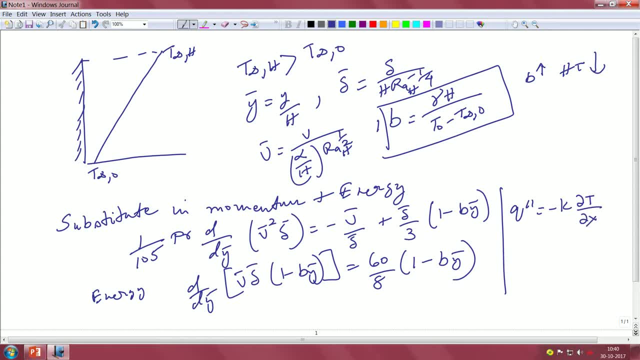 is given as k, dT by dx computed at x, equal to 0. right, that was what it was, okay. Now what will happen is that now, if you do the integration right, I mean you solve this equations, the invariant experiment- you will solve this equations. So in this way we need to find 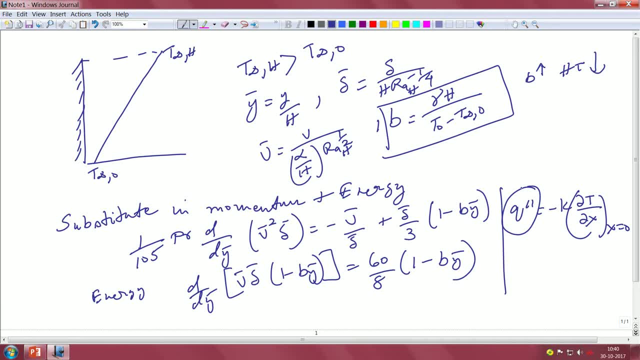 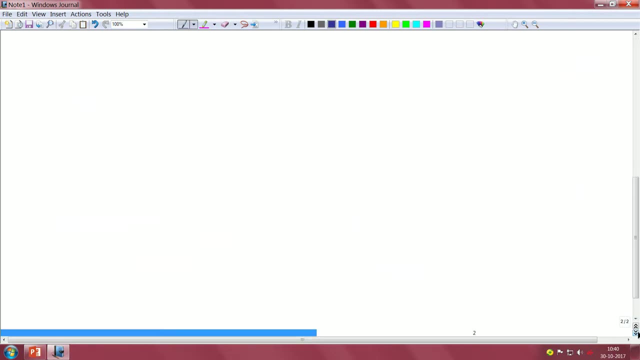 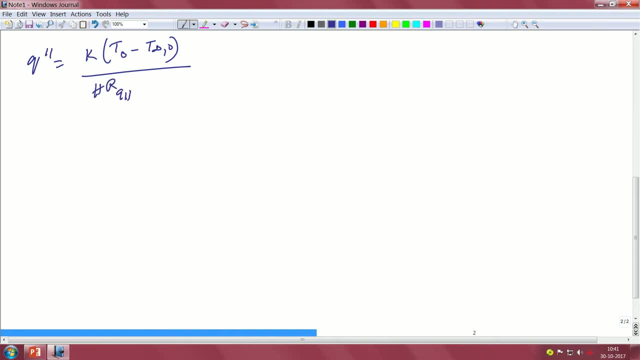 by h, r e, h to the power of minus one-fourth 2 by delta 1 minus b, y bar is delta bar. So that is the expression that you get, So naturally your Nusselt number. this is the local Nusselt. 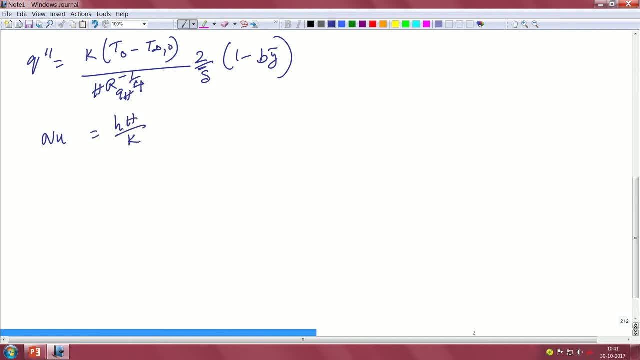 number is given by this. So that will be nothing but r e h to the power of one-fourth 2 by delta bar 1 minus b y bar. So these are the two expressions that you are going to get for Q, double prime and Nusselt number. Now the Nusselt number, of course, if you. 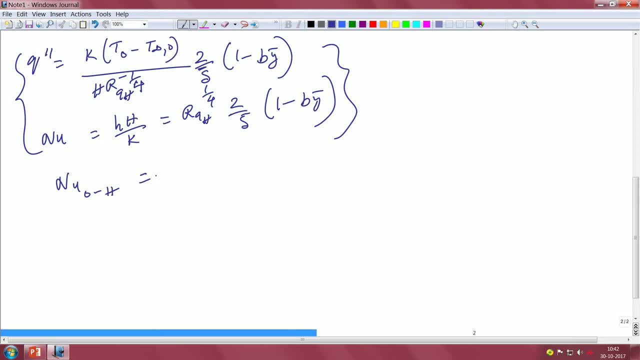 have to find out the average Nusselt number, which is from 0 to 8.. You need to basically integrate the whole expression. So this is one-fourth, to integrate it from 0 to 1, 2 by delta bar, 1 minus b y bar and d y bar. So that is the integration. 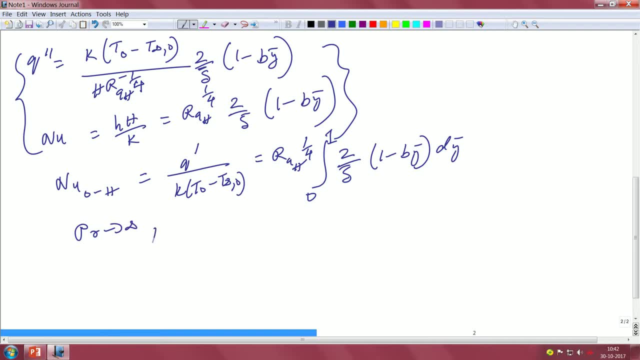 Now for Prandtl number approaching infinity. this value of the Nusselt number o h approaches something like 0.324 into Rayleigh number, to the power of one-fourth if Nusselt number approaches infinity. So this kind of this from the integral formulation, if you do more. 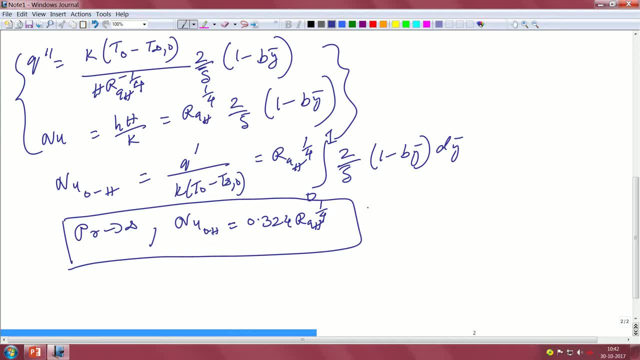 sophisticated numerical exercise on this, you will find that there is almost a 11. This is close to almost 11 percent of a more. you know what we call formidable and more complicated analytical or numerical formulation. So this is the integral formulation. So this: 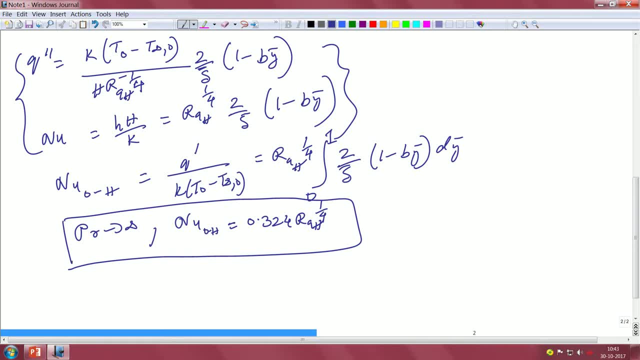 is a good way to discuss that. Now, if you look at this expression as you do in polar monochromatic formula on this particular expression, as you change b or b will change because the buenas Alcad der Carmel with respect to nusselt changes. So if nusselt number was raised, 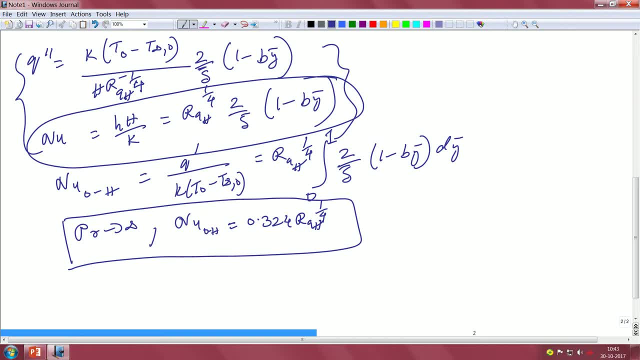 and you finished with the originalрушikka. then you just change Why? Because you had lost the original product value, right, okay. but here, however, since b is there, so depending on the value of b, your nusselt number is going to be altered accordingly. okay, so that that is the most important part. 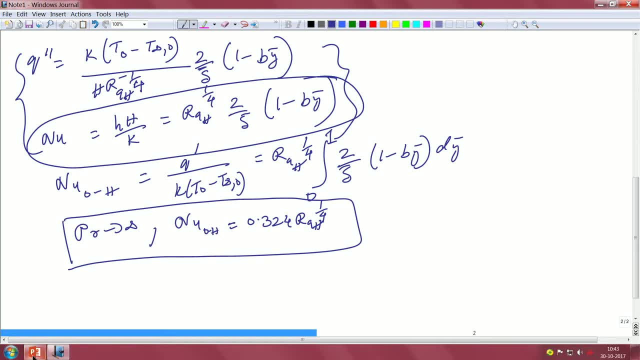 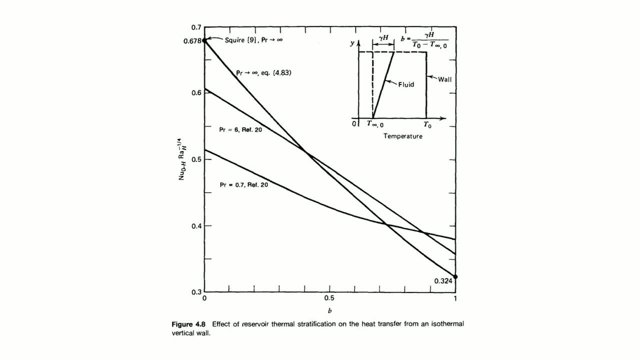 that you should kind of note. we also would like you to look at the generalized expression over here. so these are the graphs that were plotted, taken from adrian bejan. so what we can see over here, this is once again the same thing that we did. okay, so once again, you can. 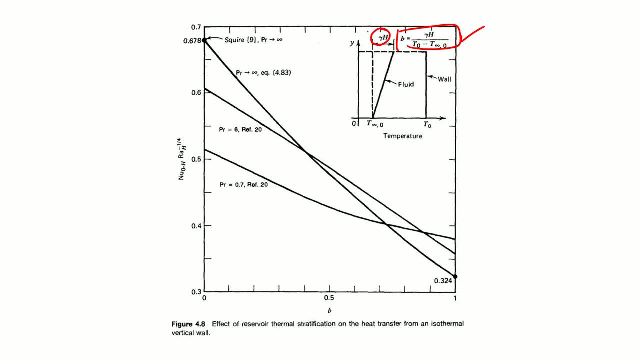 see, this is the parameter b. this is the extent of stratification. what stratification has done, okay, and what we have done over here, is that we have taken the nusselt number average and we have multiplied it out by the relay number to the power of minus one-fourth. so 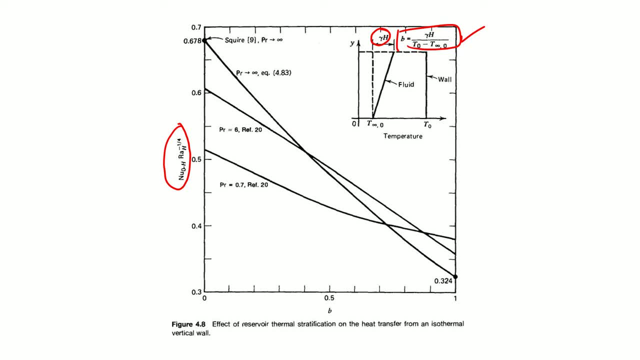 you will be left with, basically, whatever is the b dependent term, b and y dependent term, right, okay, so that is then we have plotted it versus b. okay, so, as you can see, when b is equal to one, okay, let's say. let's say b is equal to one. okay, let's say b is equal to one. okay, let's say: 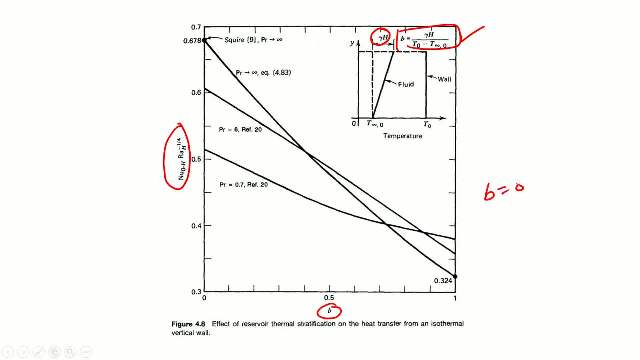 let's take first b equal to zero. b equal to zero means there is no stratification at all. okay, so when b is equal to zero, you basically get back all your original settings. right, what you had earlier? right, those were the graphs that you had earlier, right? but as we 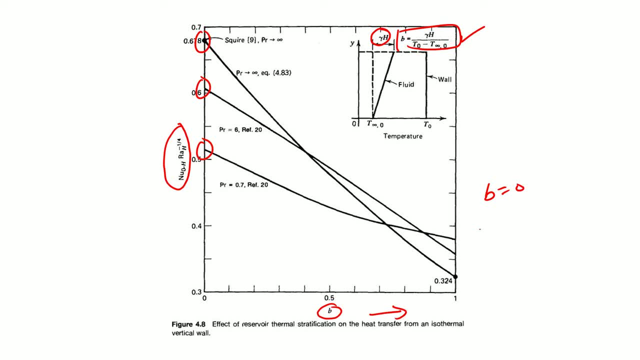 move on to b equal to one- okay. b equal to one- okay. so that means higher and higher values of b- okay, which would imply that your gamma that you have pointed out over here, that is that- is going up. okay. that means the slope is actually going up. that means this extent. 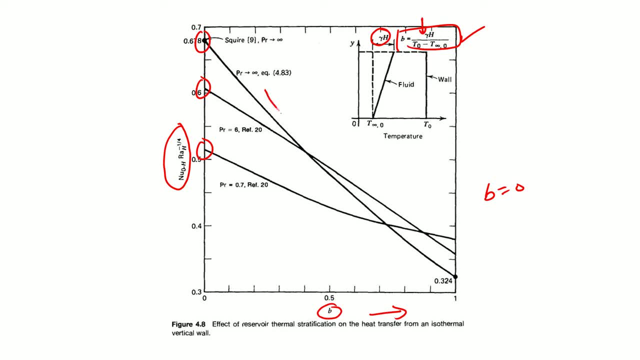 of stratification is increasing quite a bit. so naturally you see that there is a decay in your nusselt number value, which is kind of expected, right, so for prandtl number approaching infinity. this we already said was about point three to four. right, okay, for all the nusselt. 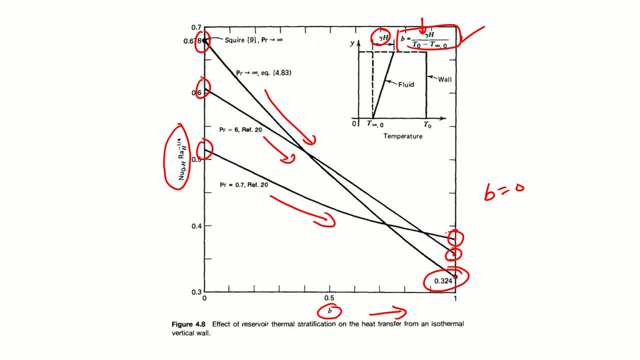 for all the prandtl numbers, this particular value actually comes down quite a bit, as you can see, from six, seven all the way up to about point three to four. so it is a loss of almost half the value, right, so all the graphs actually show that for several orders change. so this: 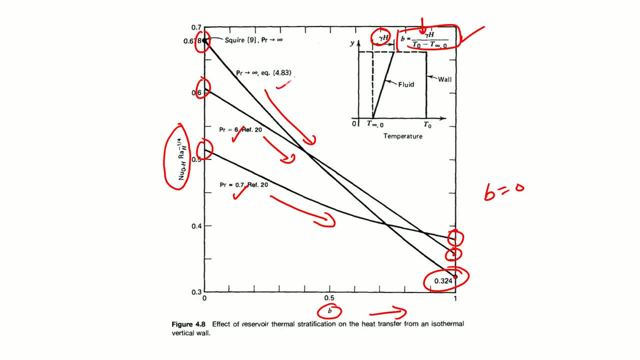 is nusselt number point six. so it is one order, this is six and this is infinity. okay, so all of them show that this is how the numbers actually decrease, but it is highly a little bit non-monotonic in nature, as you can see. 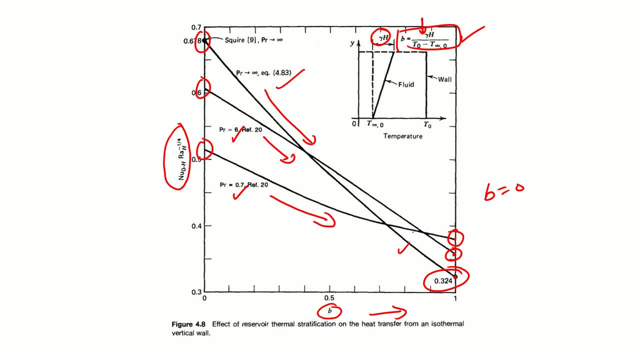 Of course, this shows the largest drop. okay, followed by this and followed by this. okay, so something that you have to there. so there is no real similarity in the pattern. per say okay, so there is a only thing that we can say: that there is a gradual decrease in nusselt. 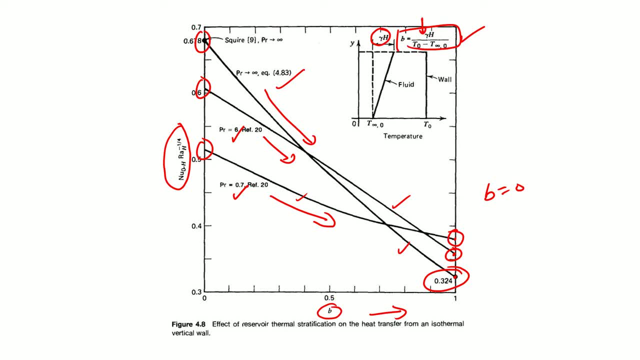 number as the stratification degree, which is b, actually increases. okay, so in the isothermal reservoir limit, okay, they fall slightly below the corollary. So in all, we can say that there is no local similarity as such. okay, but we can say for sure, as expected, that there will be a decrease because stratification is reducing the delta. 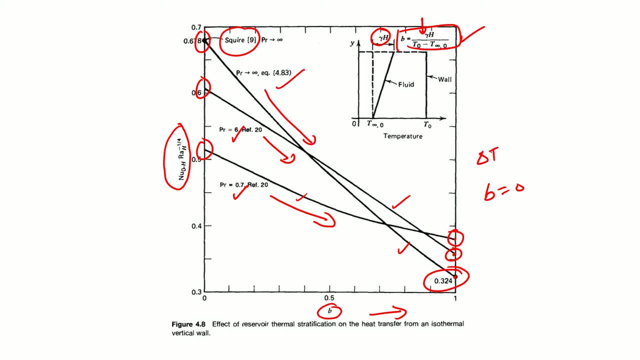 t potential, so to say, okay, it is reducing the delta t potential for this particular system. So if b, as you can see, is gamma h divided by t, naught minus nusselt, So that can be also written as 1 minus delta t minimum by delta t maximum. right, so something. 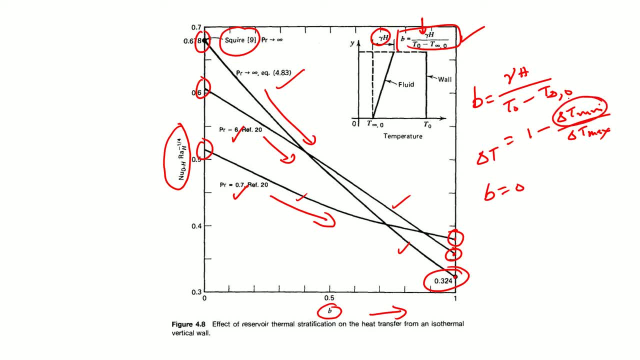 like that. okay, so as this delta t minimum actually goes on, goes on, goes on changing, right, okay, so we will have that the b parameter will increase and naturally this will hurt in the amount of heat that is coming from the wall to the fluid. okay, So this is not unexpected. only thing that is here that we have provided some fixed values. 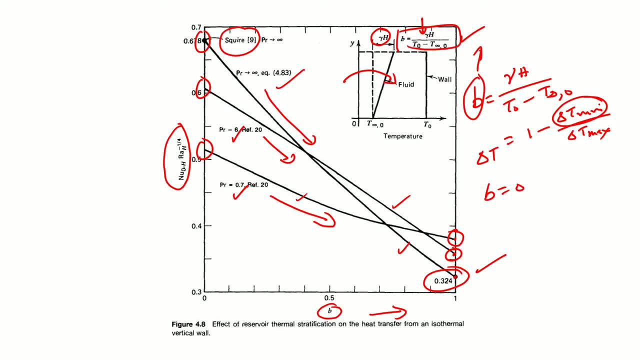 based on the integral analysis that we just did. okay, and it is like we already established that, what will be the temperature profile, what will be the velocity profile and things like that. but so it is a, it is a simple substitution, but we are able to predict the, the slopes. 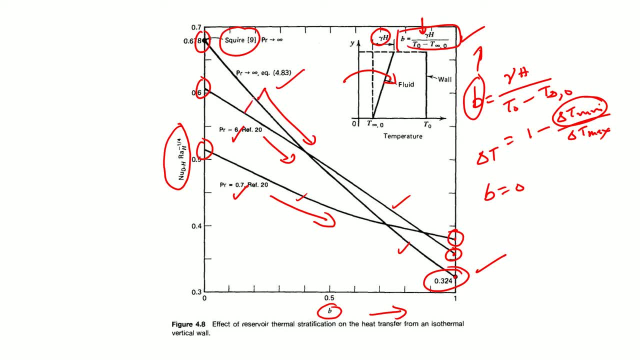 and the slopes are not like they. these might look a little linear. this is this: looks like this has got some kind of a parabolic or a power lock. Okay, So it is a kind of dependence, or polynomial kind of a dependence, in this particular case. 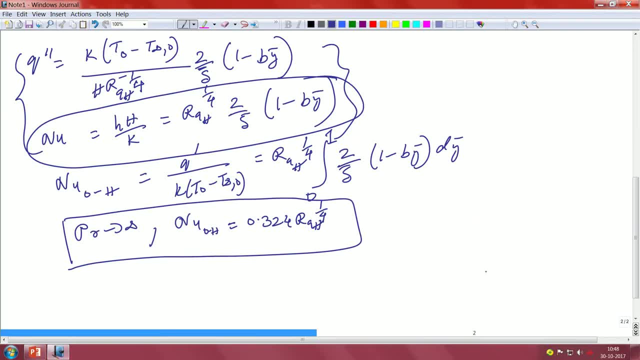 okay, so let us move to the other one. so, based on this, it is quite obvious now that we have been able to say that. what would so just remember these values? this is the local nusselt number, okay, and this is basically the average nusselt number, so these two things must be kept in. 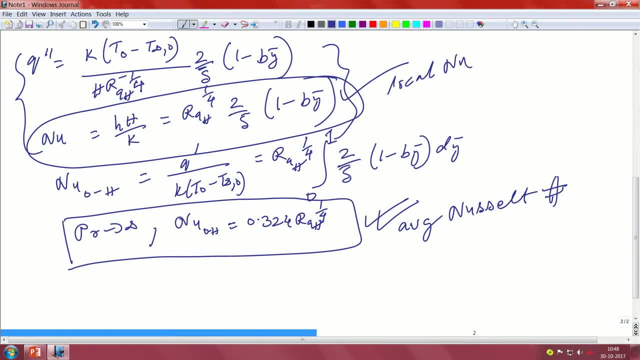 in your mind When you actually attack the problem. okay, so let us now look at the situation where the two vertical walls are basically a little bit closer to each other. so this problem is an interesting problem in the sense that it is, it is applicable in a wide variety of applications. 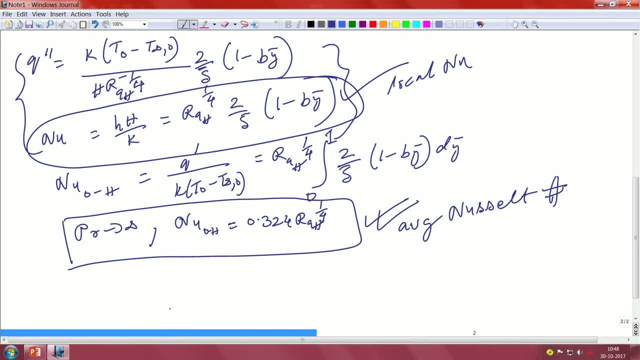 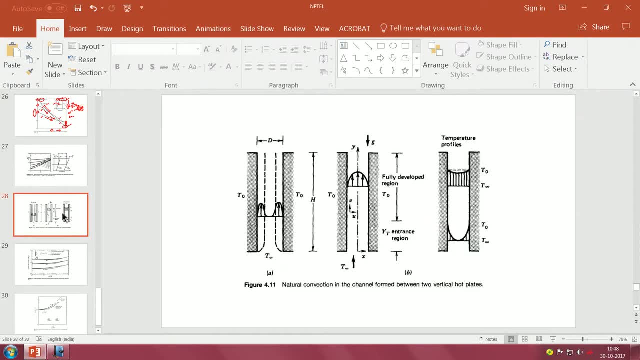 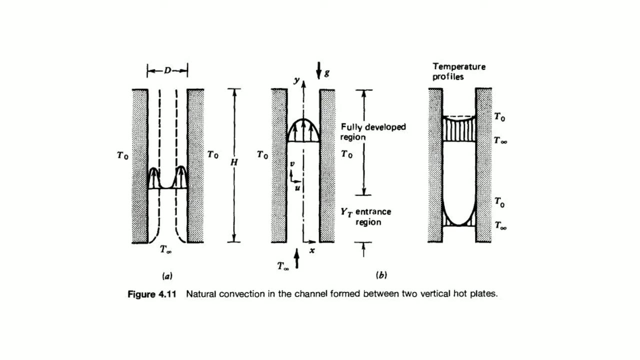 ranging from fins, electronic cooling- okay, because where the two walls- I mean the two fins- may be placed very close to each other. so, before looking at it, let us look at what I am actually talking about. So let us look at this particular profile, okay. so, as you can see that this is the normal, 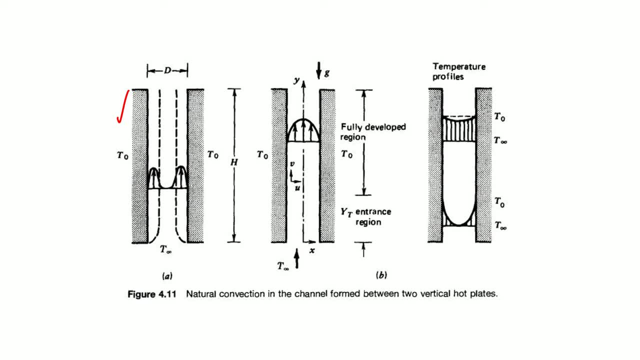 vertical wall that we were actually dealing with, right? what happens if you place another vertical wall right next to it right now? if the distance between the two walls, okay, is much, much greater than the thermal distance or the thermal boundary layer thickness, which is delta, okay, delta t or delta? 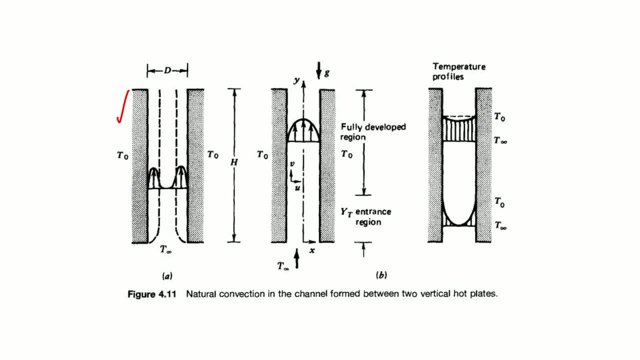 Okay, Okay, whatever you call it. okay, if they are sufficiently- if this they have, they are sufficiently placed far apart. okay, so what do you expect to get? you expect that these two velocity profiles, okay, will remain almost distinct with respect to each other right throughout the length through which the traverse. so these are the wall jets, right? 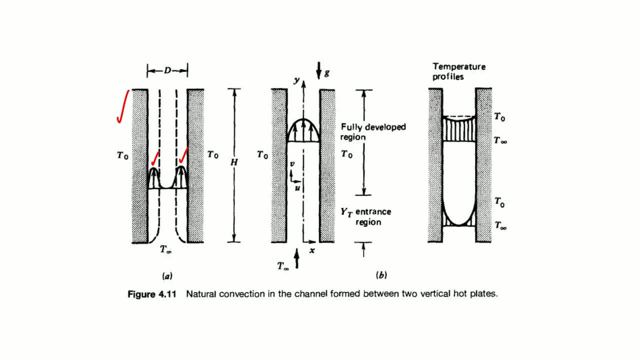 So these wall jets will remain distinct from each other, very distinct from each other. they will not cross talk with each other because of the simple reason is that the distance between the walls is sufficiently far apart. they are, they are actually sufficiently far apart. okay, Let us look at the scenario two, when the distance between these walls are very close to each. 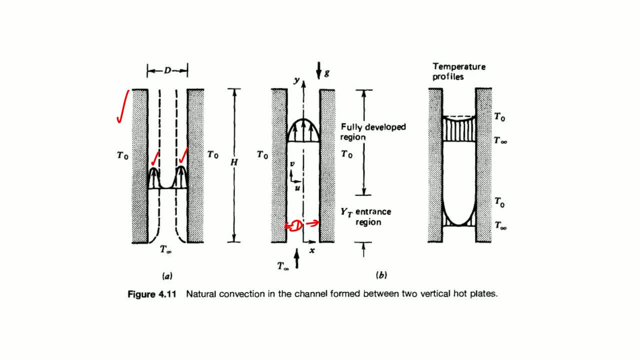 other. right, they are very close to each other. that means these two velocities will now start to cross talk. okay, So the Okay. Okay, They will kind of merge right and you get a very similar velocity profile, like what you normally expect in a duct right in the forced convection paradigm. okay, so the flow. 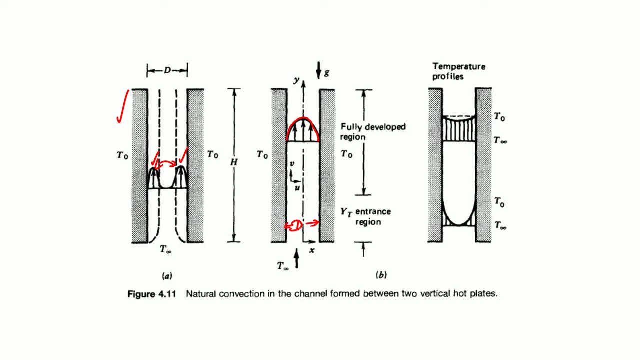 will be like that: okay, there will not be any distinct. you would not be able to distinct the two wall jets. they are basically cross talking with each other. okay, and similarly, so you can see what happens when you actually have the temperature profile distinct versus not so distinct. okay, 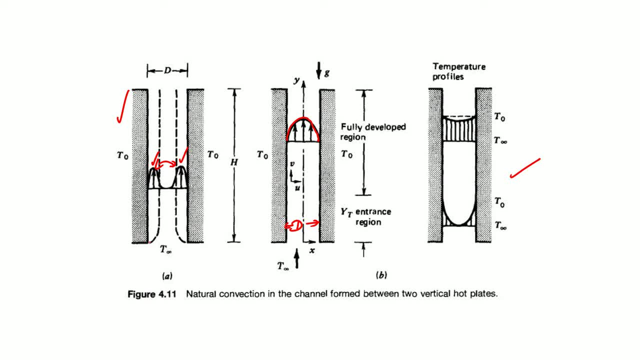 So in these cases- Okay, You know that the boundary layer takes a little bit of time to develop, right? that is the same as in the case of a pipe flow or any other flow, right? the boundary layer takes a little bit of time to develop. so there must be some kind of an entrance length right before these. 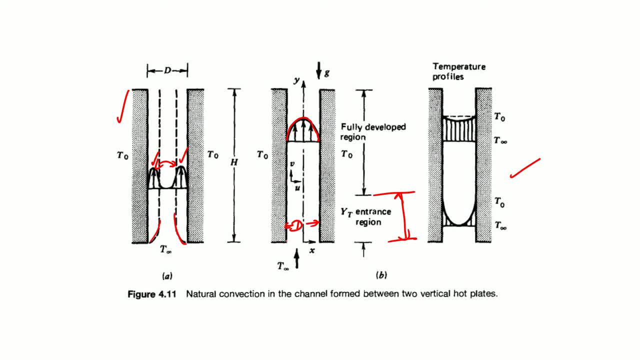 two layers actually merge with each other must be okay. So you mean to say that there should be something like this, probably right before these two layers actually merge with each other, and that merging length is given by this parameter right, This parameter which we called as y t right, since y t is the parameter which governs this? 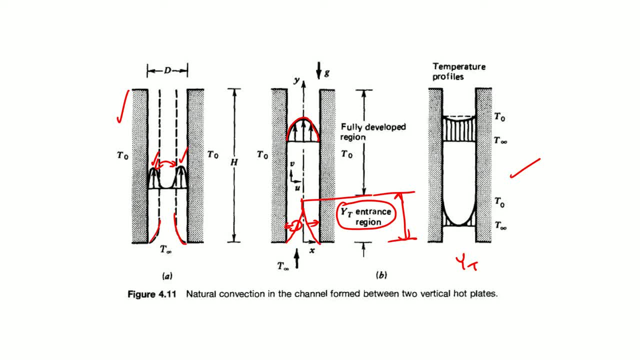 okay, so let us now see that how we can analyze the problem in the case of a duct flow. remember it was a pressure driven flow, so there was a pressure head which was actually maintaining the flow. right here, of course, it has to be the temperature difference, so the temperature. 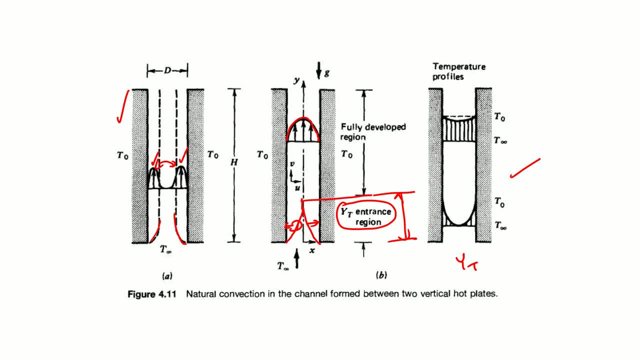 difference creates a flow which resembles- which kind of mimics, right- what we actually see in a In a In a duct. okay, and actually whether the velocity profile will be parabolic or not, that we will see shortly. but in a nutshell, if these two profiles merge, they will look something like: 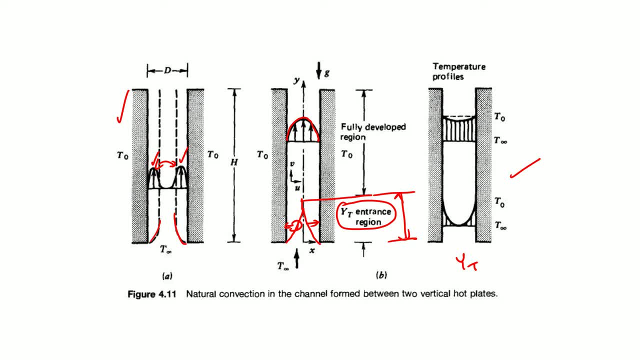 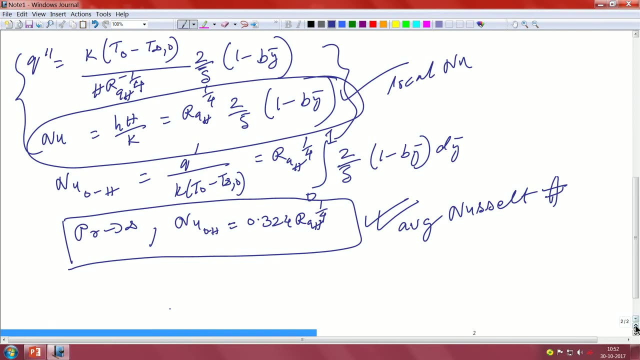 that right, but there would be similar to the forced convection counterpart. there will be some kind of a, you know some kind of a merger of the two layers, and we will see how to analyze a problem like this. okay, So let us go to our little notes. 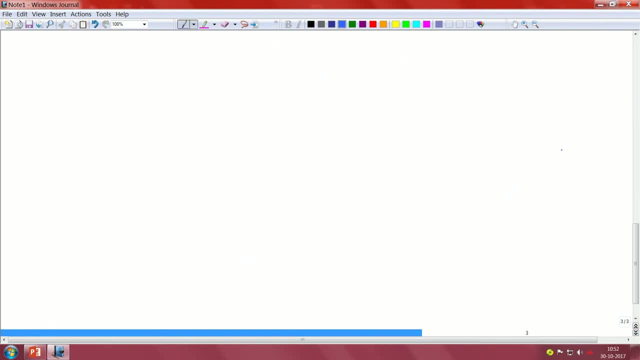 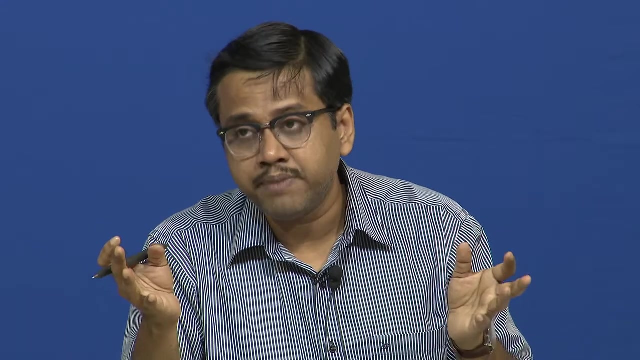 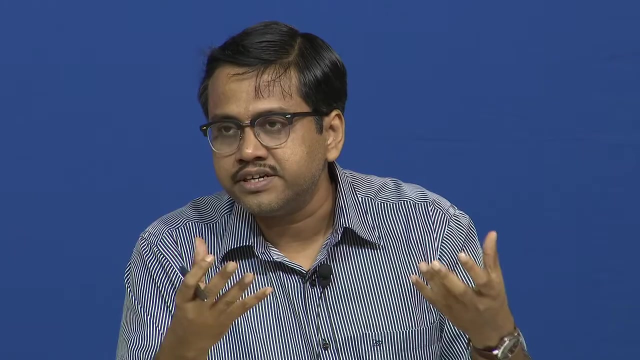 Now so, having laid down the problem, and this is widely used in the case of electronic cooling and things like that. in fact, this is one of the key pieces of design parameter that one would normally use, because when you try to design a coolant, cooling circuit, right fins, 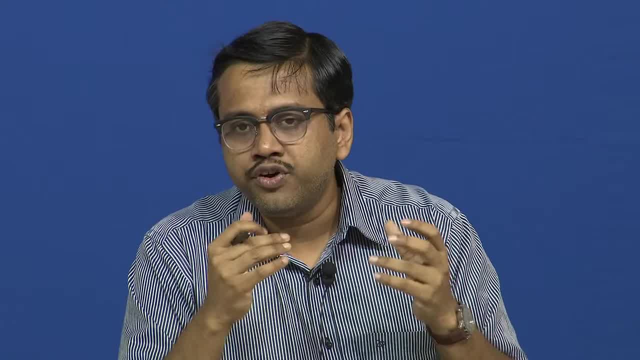 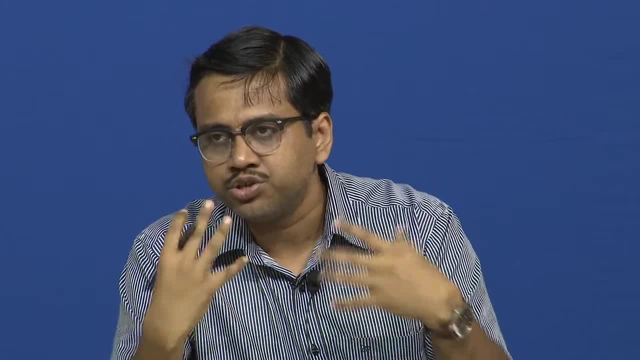 especially in your computers and other things, okay. Okay, If you are relying on forced convection to do the effect, then how these two layers are cross talking with each other and how the heat is actually transported, it forms a large part of the problem, okay. 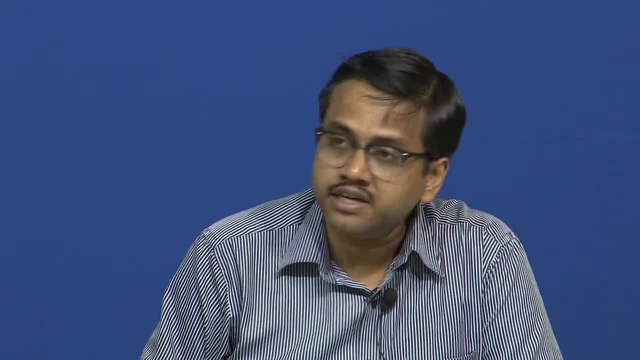 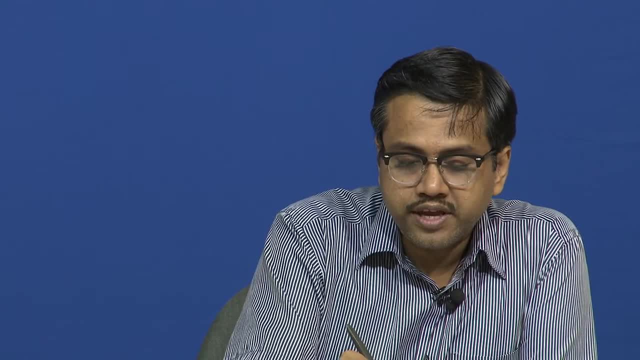 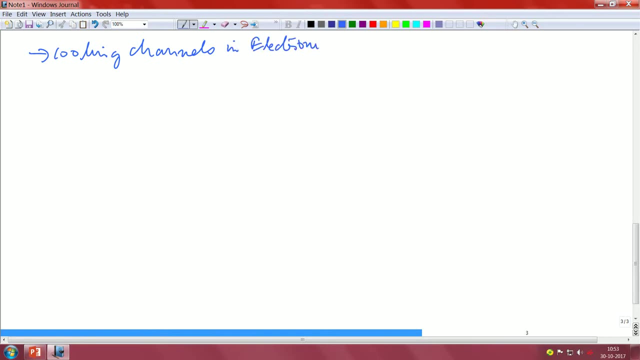 So it is very characteristic of vertical, fin to fin cooling channels. okay, in electronic equipment. remember that in mind. okay, So cooling channels, cooling channels in electronic equipment. in electronics it can be in other cases also, especially these era of, you know, micro scale cooling or micro cooling. okay, 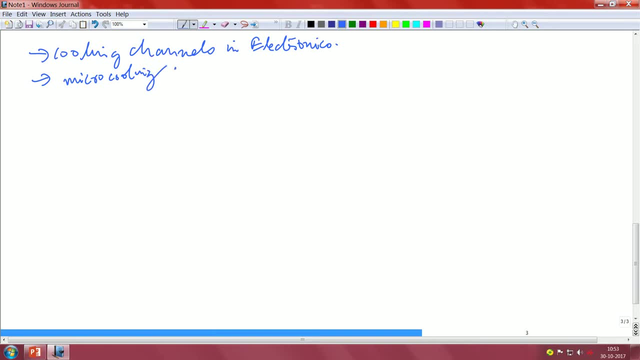 All those things can be very important, okay, and micro cooling, using, you know, micro to mini channels- these are all very, very, very important over here. okay, Now, let us now take the, the flow part and try to analyze the problem. okay, In a So, the. so the problem essentially boils down is that this D, which is the separation between 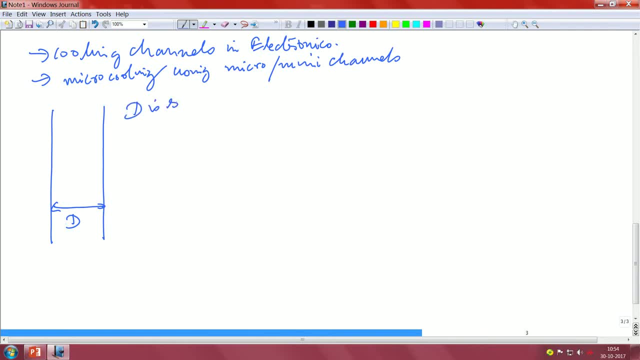 the two plates. okay is small, D is small, okay, and if this is the axis, let us define the axis. this is your x, this is your y, so this is naturally. this portion is basically D by 2. okay, and obviously these two layers merge with each other. all those things are very similar. 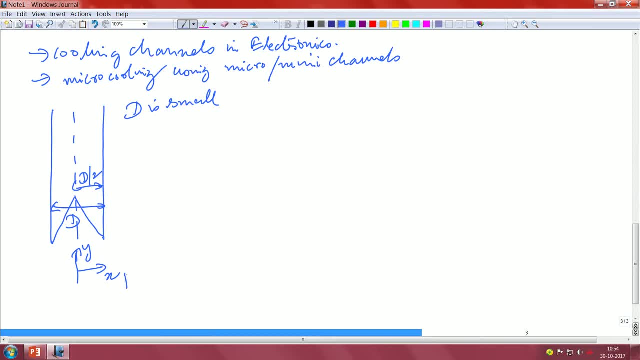 to the pipe flow situation. Okay, So this is given by u, this is given by v, right, so that is the. that is the way that we have always defined it. So the momentum equation: if we write the momentum equation, okay, it will be rho dx plus v dvdy. 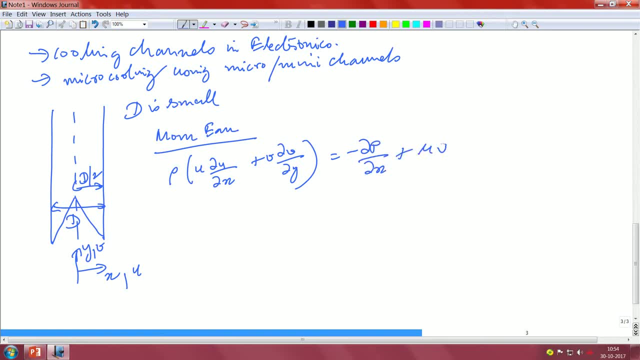 minus dp, by dx plus mu, Right, this is the momentum equation. so, similarly, looking at this particular kind of a velocity profile, what we showed, right, like that, right, we showed the velocity profile. of course, this is the peak. okay, the velocity profile that we showed, okay, we can safely assume that, perhaps, 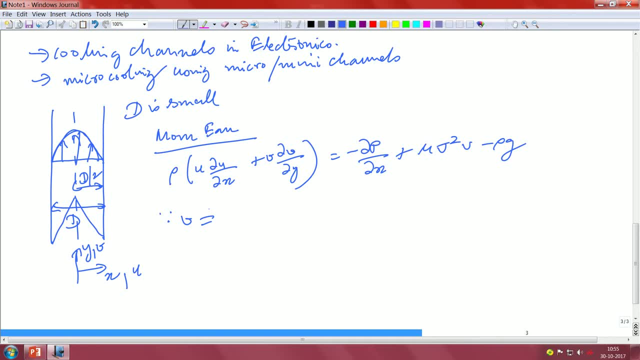 your v, that is, the velocity in the vertical direction, is not a function of y. it is very similar. Now you could generally say that phi is the velocities. Bye bye, Bye bye. This we already established earlier. It is like a hydrostatic head that we develop. So 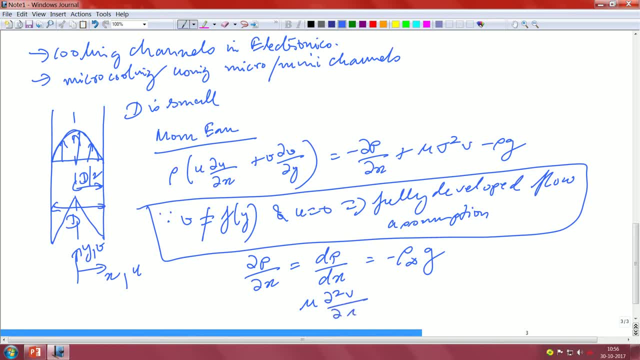 this will become. that is the only term that is remaining. So there is, of course, gravity here, because gravity is always important in this. So, as you can see, of course there is no pressure gradient, but you have this hydrostatic and this buoyancy driven flow. 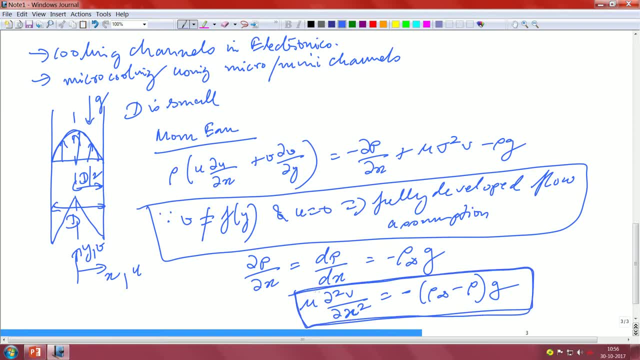 essentially, which is basically trying to balance This viscous term. this is nothing but the viscous term. Very similar in origin. very similar how we have actually analyzed the problem that v is not a function of y and u is equal to 0. This is our standard definition of fully developed flow. That means the flow. 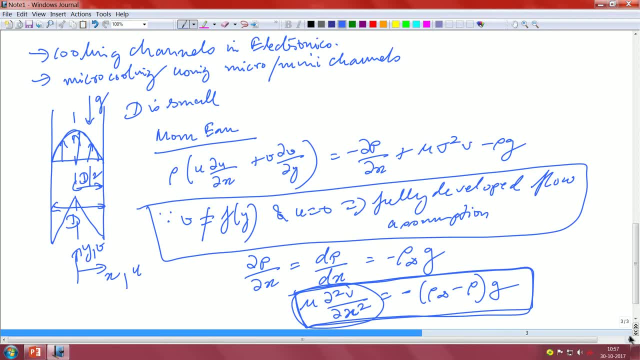 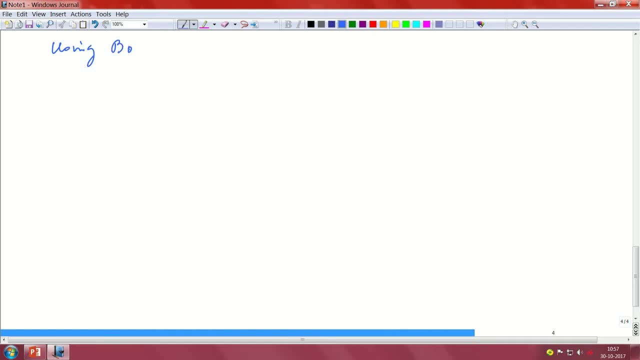 is convectively non-accelerating. So that is what we did earlier. Now, using our Boussinesq's approximation, if you recall the Boussinesq's approximation where we said that in the convective part. 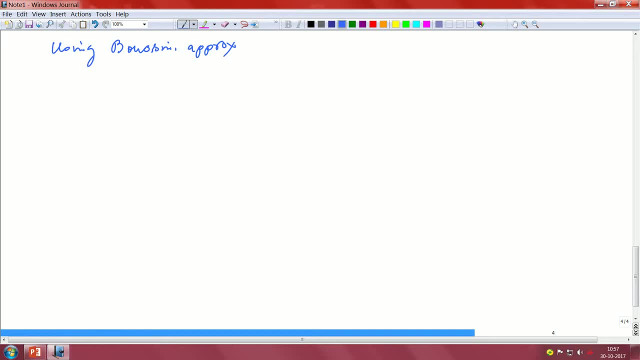 it is usually a constant density and the variation only happens in the buoyancy part. Remember that was what Boussinesq's approximation was. So, using Boussinesq's approximation, This particular problem, therefore, we had to go beyond this. So this is a very easy, very 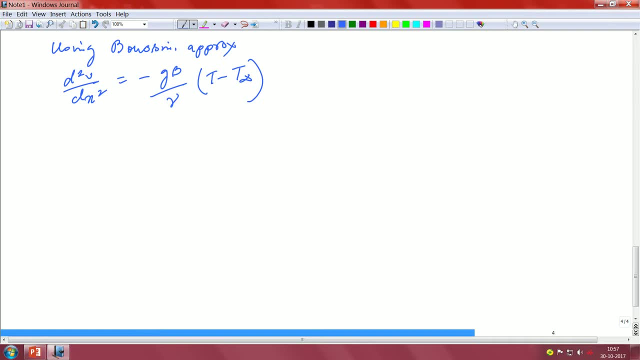 4 becomes unsolvable when you write it like this, because it is G beta by gamma into the T minus T. infinity is generally a problem which cannot be solved because you have velocity as an unknown, you have temperature as an unknown. So what we need to do is basically: 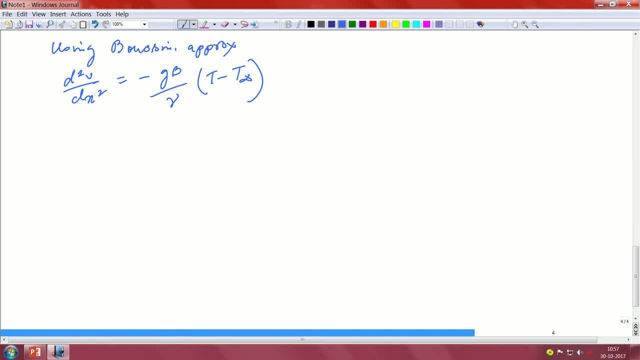 you need to couple it with your energy equation and solve it kind of together. Together you have to solve these two equations. but of course this particular expression is equivalent to the Poiseuille flow, to the Hagen Poiseuille flow in forced convection, So it is equivalent. 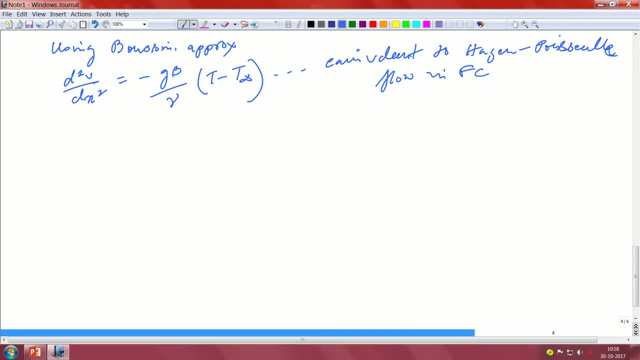 but this natural convection equivalent of the Hagen Poiseuille flow, but it is cannot be solved in such a such a nice way as we did in the case of your Poiseuille flow. So what we have done, what we can do over here, is: 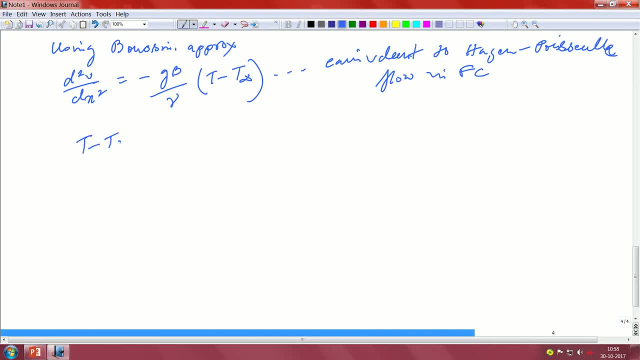 that if we assume that is T minus T infinity, we assume that this particular thing, almost equal to T naught minus T infinity. That means how, what we have done, we have got to rid of the problem of T minus T infinity and we have substituted it by a constant head. 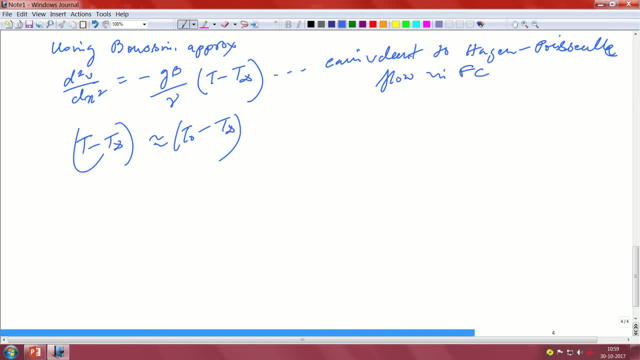 temperature difference. like T naught minus T, So this T naught minus T. that is what we have done. we have approximated the temperature difference by this. So this is approximated the temperature difference. So moment we approximate the temperature difference, then the problem becomes solvable. 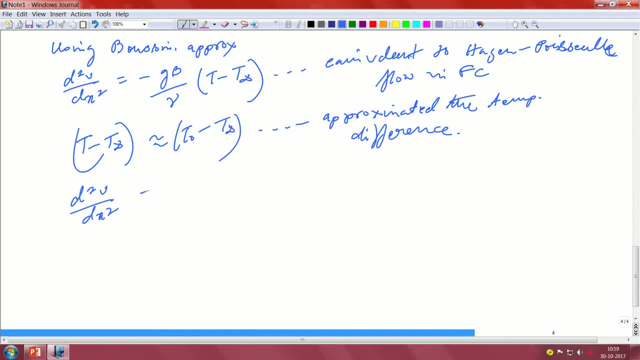 that is because your equation now boils down to minus G B, gamma T naught minus T infinity. So you can apply your first integration. this is G beta by gamma T naught minus T infinity. G is basically calling for the T set of deliveries, So neg 빼 D star will be T plus zeta. Now let us make 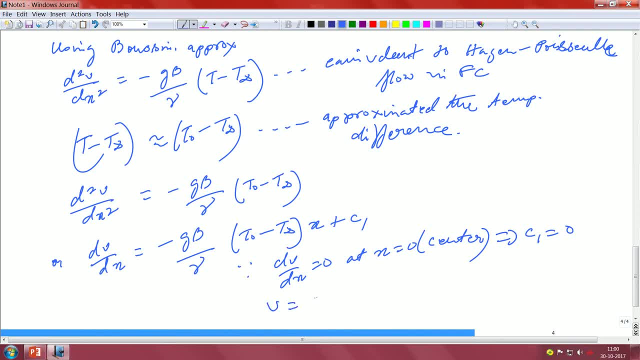 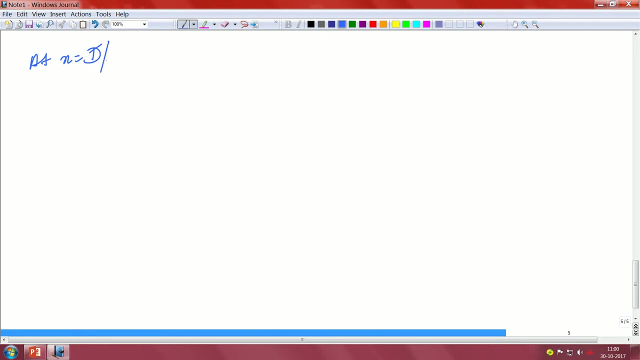 this equal to 0.0.. So therefore your V now becomes G beta T naught minus T infinity, divided by gamma, x square by 2 plus C, 2.. Now, at x equal to D by 2, that means at the wall, your V should: 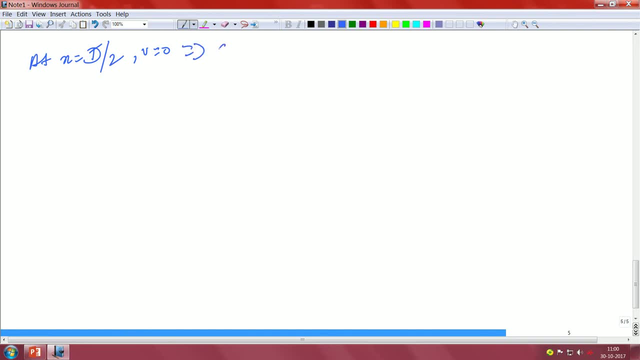 be equal to 0, because of the no-slip condition, This leads to your C 2 to be equal to G beta T naught minus T infinity, divided by gamma x square by 2.. So your velocity, therefore, your velocity becomes G beta T naught minus T infinity divided by 8 gamma T naught minus. 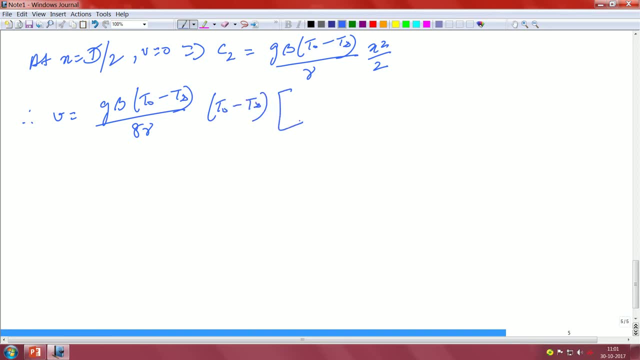 T, infinity, And there is a D square here. So in this particular case, as you can see, this is basically the driving mechanism. This is basically what is your driving mechanism. So, like in the pressure head we had, in this particular case, this is basically the driving. 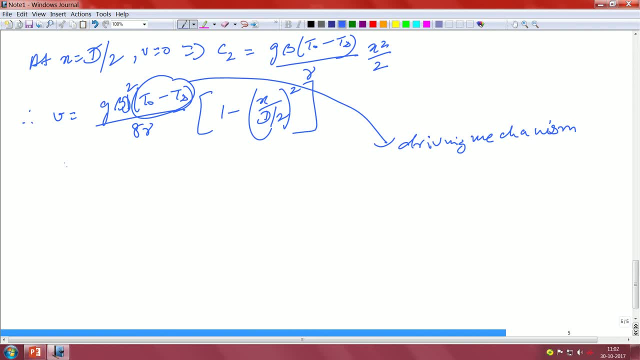 mechanism of the flow. So we have established what is the velocity scale going to be. Now it remains to calculate the 27.6 ót per m meter square. The work we are doing now is calculate what is the corresponding heat and what will be the corresponding, you know. 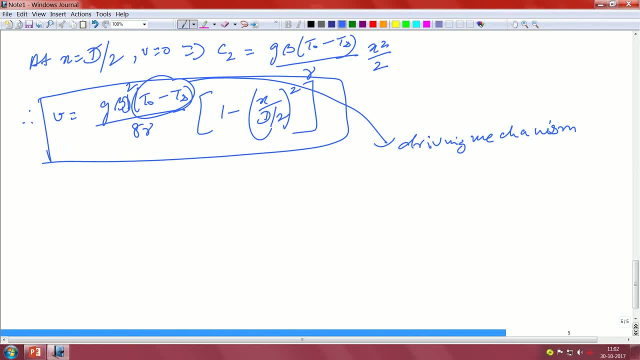 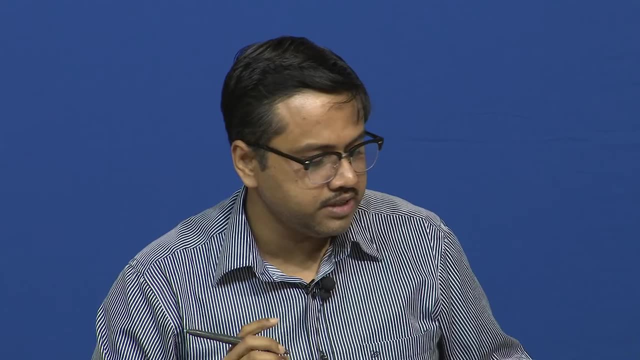 the Nusselt number and stuff like that. So let us look at that in the next class. So here we have established up to the velocity scale of the problem. So let us see that, how the Nusselt number and the heat release comes into the picture when the two plates. 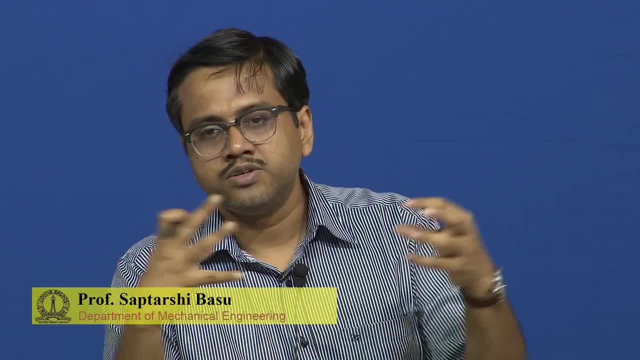 are very close to each other and they are cross talking with each other, So that the two flows have basically merged with each other. thank you.